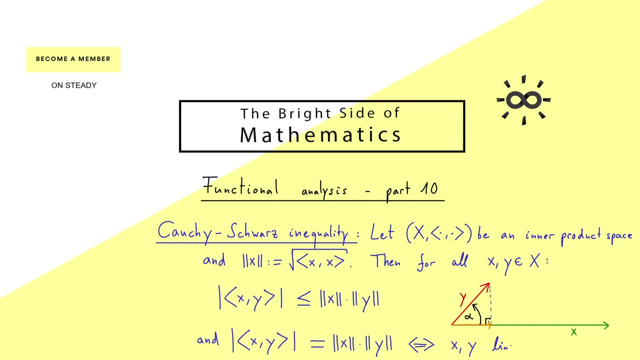 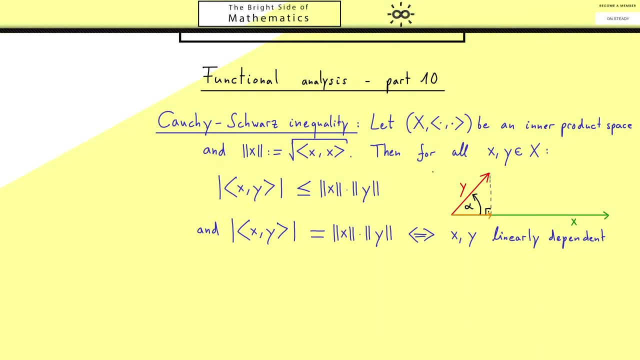 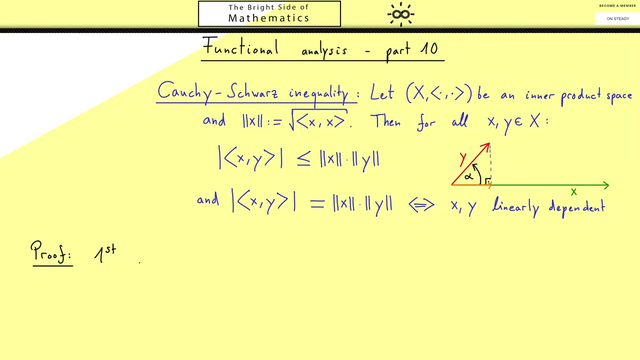 In other words, x and y are linearly dependent vectors. Okay, now the picture gets us in the correct direction, but we don't have any choice. We need to prove the inequality now. Okay, so let's start with an easy case. Let's call it the first case where x is the zero vector, Of course there. 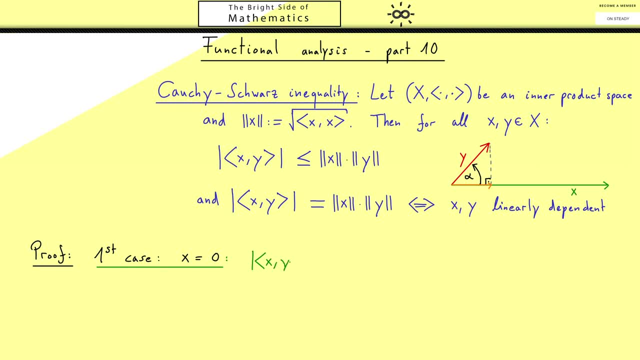 we know, the left hand side has to be zero. Simply by the linearity, we can just pull out the factor zero. And of course the right hand side is also zero because the norm of x has to be zero. here In particular, the general inequality is obviously fulfilled for this simple case. Now you might already guess the actual. 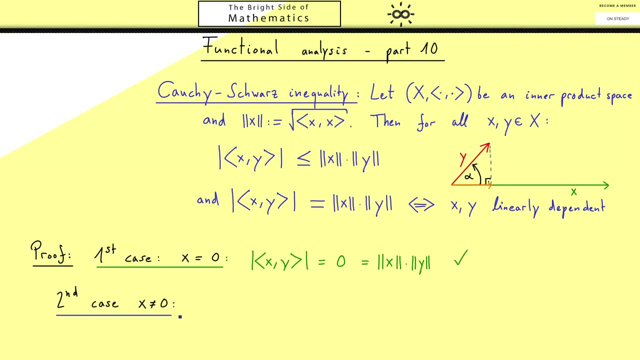 interesting case would be the second one Here. x is not a zero vector, which means we can divide by the norm of x, And that's what we do immediately. I want to define x hat as the normalized vector x. This means that x hat has length 1, so it just gives the direction of the vector x. 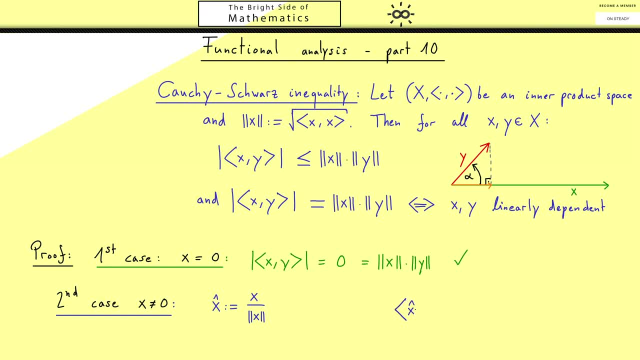 And then we calculate the inner product with x hat. We calculate the inner product with x hat and y and go into the direction of x hat. Now you might recognize that, because if we have considered the normal Euclidean geometry in the plane, this picture would be completely correct and this expression is exactly this orange line. 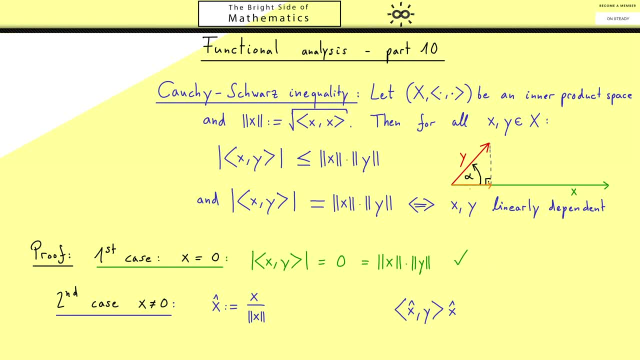 By our abstraction. this should be the same here. so let's call the orange error just y parallel. In the Euclidean geometry this is known as the orthogonal projection of y on the left to x. So it makes sense to do the same for a general inner product. Now the 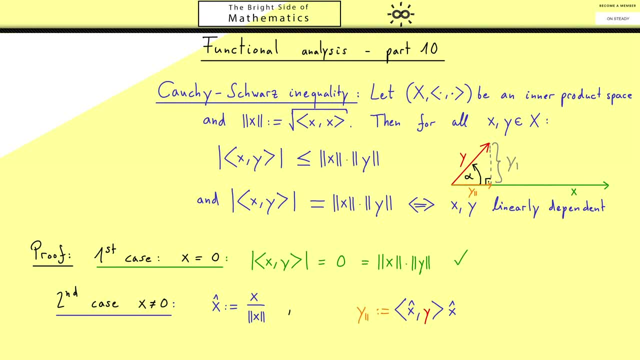 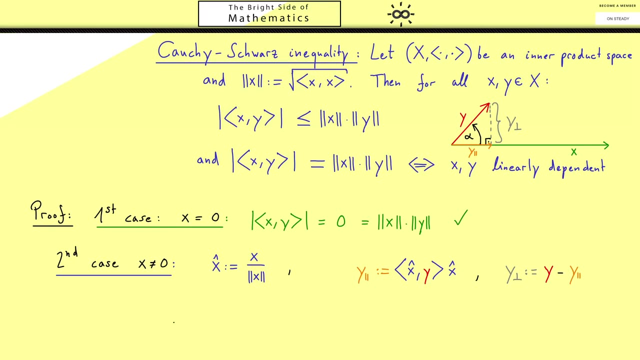 gray line. here is the orthogonal part, which we also can calculate. now, This is simply given by y minus the parallel part. Okay, so we defined some vectors we want to deal with, but now we need an idea how to get to the inequality Indeed. the whole idea is that we can calculate the length or the norm of this. 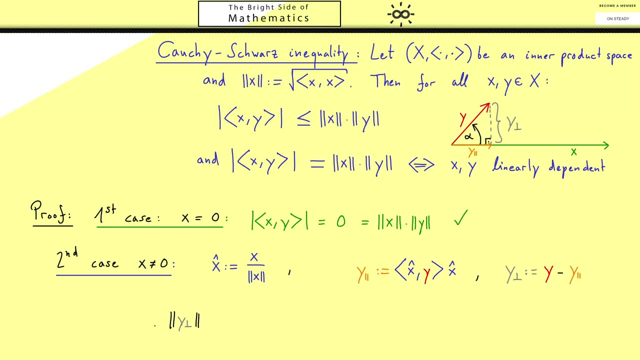 orthogonal part, Simply because we know the norm can't be negative. Now, on the right, we can put in the definition and then of course also the definition of y, parallel. Now, if you see something like this, calculating norms but you have an inner product, it's better to use squares. So square everything and the square. 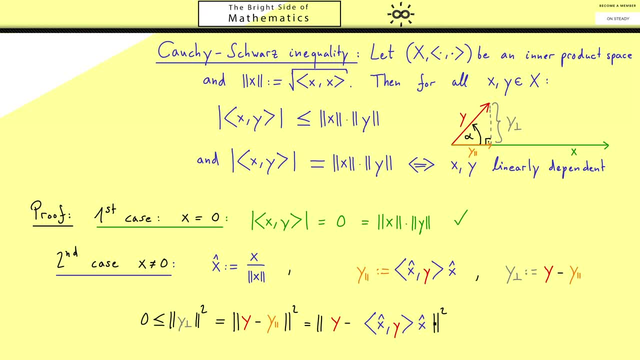 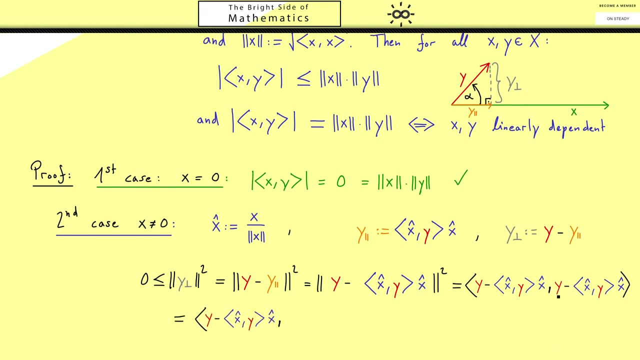 roots will vanish And now you can see, on the right hand side, we have this long vector In the middle in both components of the inner product. So it looks like this And in order to simplify this, we will use the linearity And this linearity in the 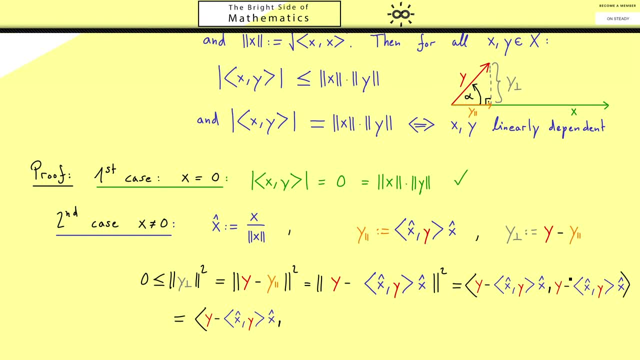 second component means we can pull out this minus sign here. So we have here the inner product with y minus the other part. In the next step we want to pull out the minus sign here and here, And we know we can do that because the inner product is. 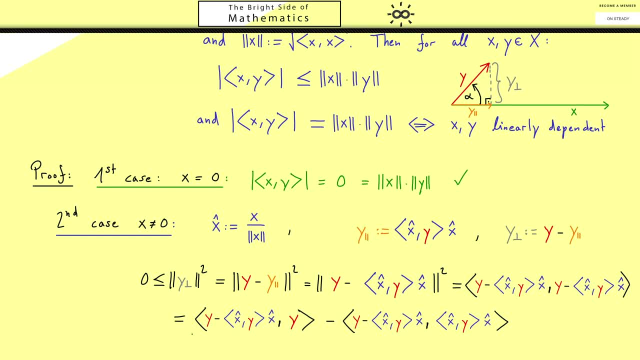 conjugate linear In the first argument. So minus signs are not a problem and scalars get a complex conjugation. So that's the first part, and the second part would be this vector with y, And of course now we do the same with the second inner product here. 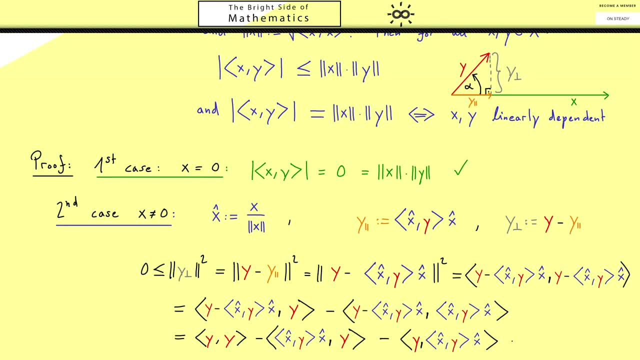 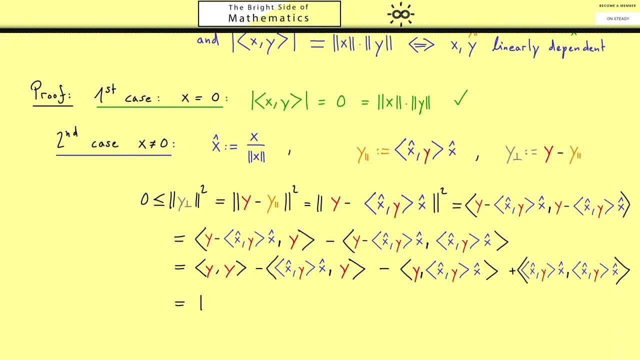 Okay, here we have y with the vector on the right hand side, and now we have minus, minus, so plus the rest. In fact, here we have the same vector left and right in the inner product. Therefore, now comes the part where we can rewrite everything again. The first thing is the norm of y, squared For the 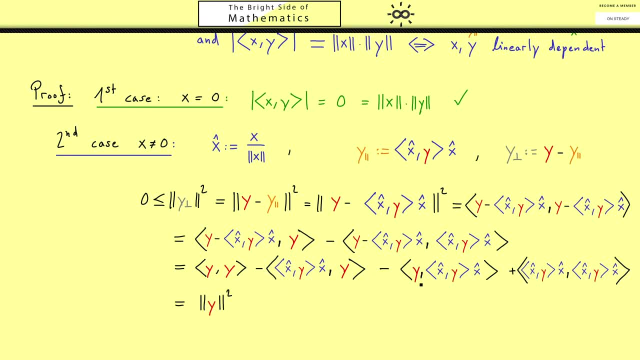 two parts in the middle we see they are almost the same. The one is the complex conjugate of the other one, So we can write it in this way, with parentheses where I put a bar over the second part. And finally, the last part is the norm of: 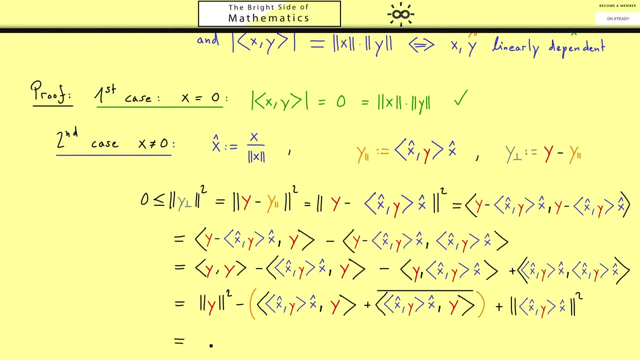 this vector squared In the next: equality. here I want to simplify that even more because you see, here is a complex number plus the complex conjugate of this number, number, which means this is 2 times the real part of this complex number, Which means that we can write it like this: 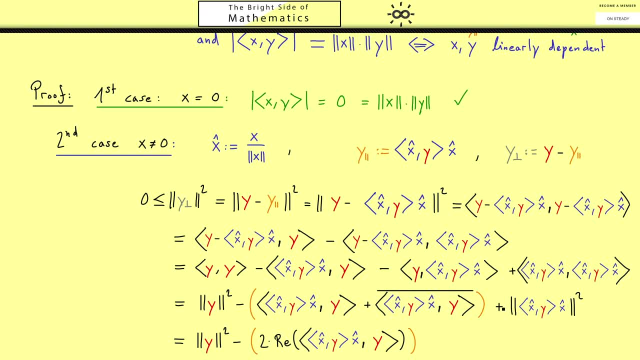 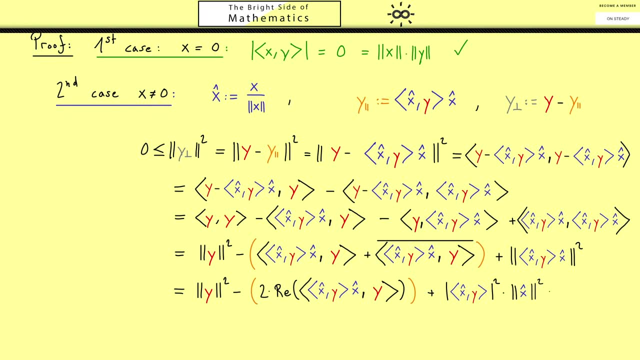 And now, in the third part, we can pull out the scalar, which means it comes out with the absolute value squared. You see, it remains the norm of x hat, where we already know this is 1.. Now, finally, I want to simplify the middle part here which, to be honest, we could have. 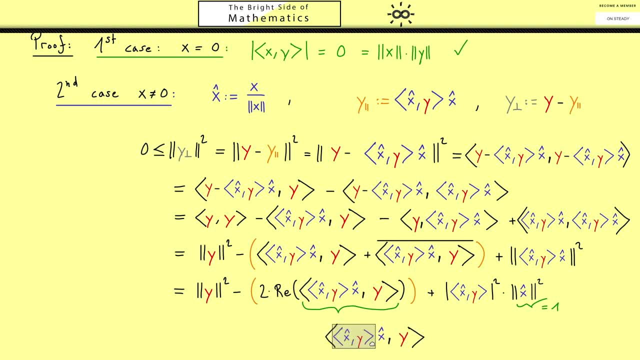 done before, but then we would have done it 2 times. I want to show you visually what we want to do. we pull this scalar out from the first argument of the inner product, But then it gets a complex conjugation. So let's fill in the gaps again and then, you see, we have the same complex number left. 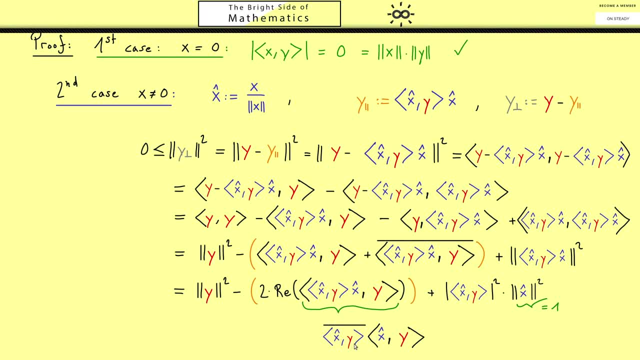 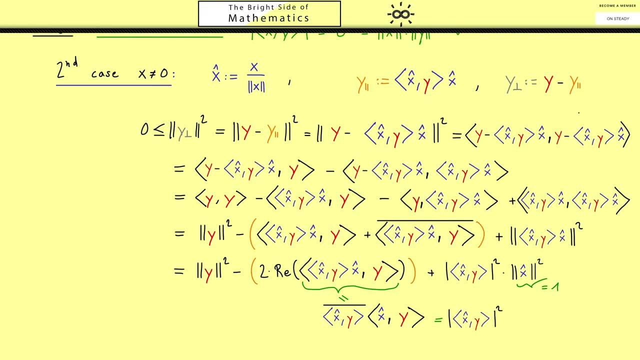 and right, but the one is the complex conjugate of the other one. In other words, it's the absolute value of the complex number squared, And since that is clearly a real number, we can omit the real part here. So, in summary, 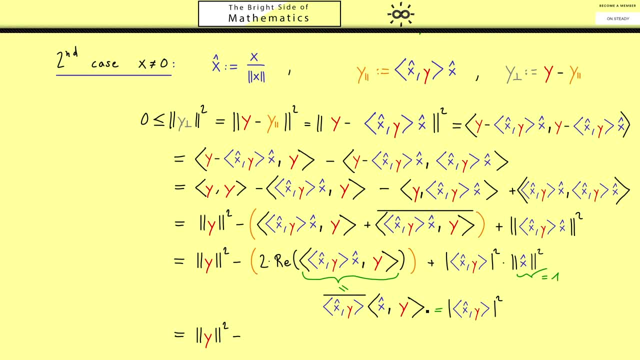 We have the norm of y squared minus 2 times this number, But also plus 1 times the same number. Therefore we can put both things together and have a simple result here: The norm of y squared minus the inner product in the absolute value squared. 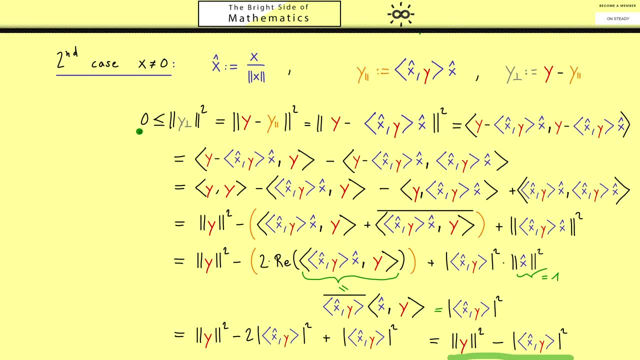 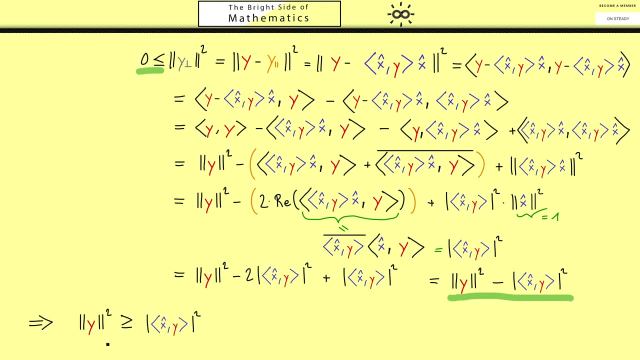 So this is our right hand side, and on the left we have the zero Hence. in the next step, I want to bring the inner product to the other side. Now you can see, We are almost there with our inequality. the only thing missing is that we have to translate. 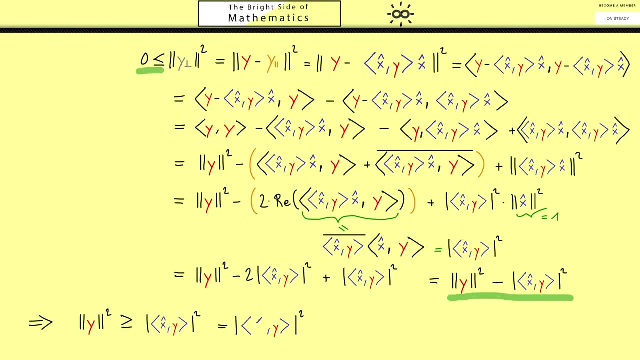 back x hat, Which is not so hard to do because we define it as x divided by the norm of x. Of course, we do the same as always: we pull out 1 divided by the norm of x. Hence, that's what we get, and you see, we just have to multiply with the norm of x squared. 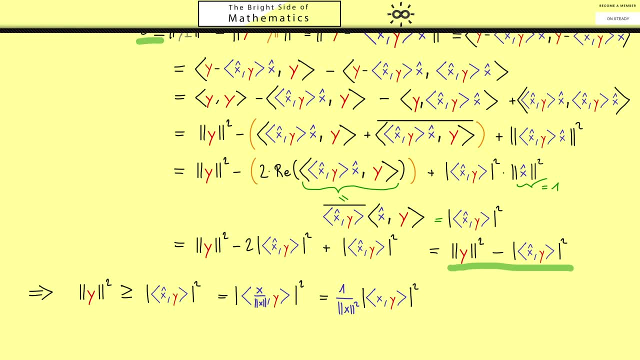 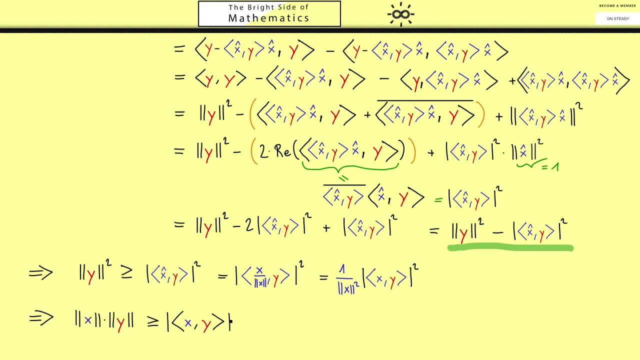 on both sides And then, taking the square root on both sides, we get out our Cauchy-Schwarz inequality, And that's it. Well, that's the whole proof of the inequality. I will skip the part about the equality now, because I want to use the time to show you. 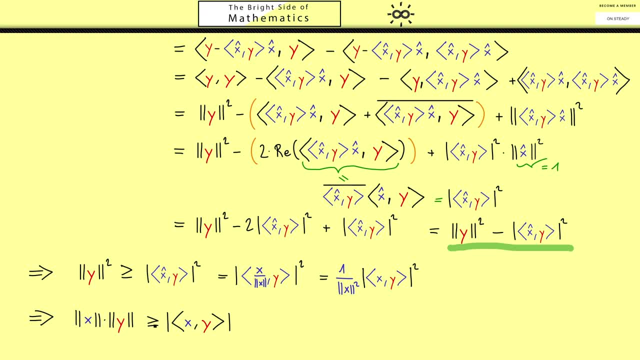 that the symbol we use here is indeed a norm, so it fulfills the triangle inequality, And we will do that by using the Cauchy-Schwarz inequality. In fact, the triangle inequality is, most of the time, the hardest part of a proof that. 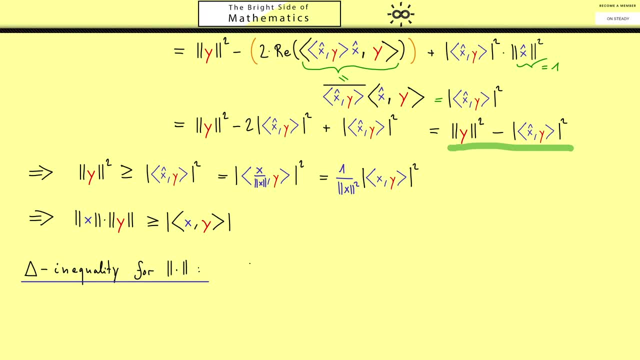 something is a norm, So let's do that very quickly. Of course we square the norm again, Because then we don't need the square root. we can just write x plus y, x plus y in the inner product. The linearity now gets us to a similar result as before. 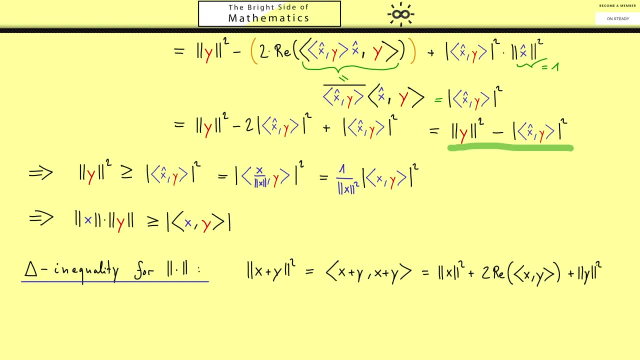 Namely the norm of x and y squared, and in the middle we get 2 times the real part of the inner product. Now, of course, if we use the absolute value instead of the real part, it gets bigger. And of course, here we now can use our Cauchy-Schwarz inequality.